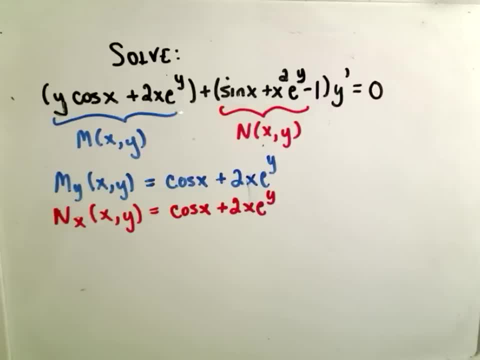 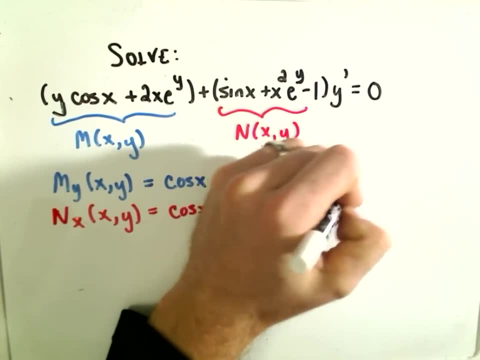 And the minus 1 goes away. So, hey, these are equal to each other. This now is 2x. This now tells us that this equation is exact. Okay, Okay. so now the next thing that we want to do here. 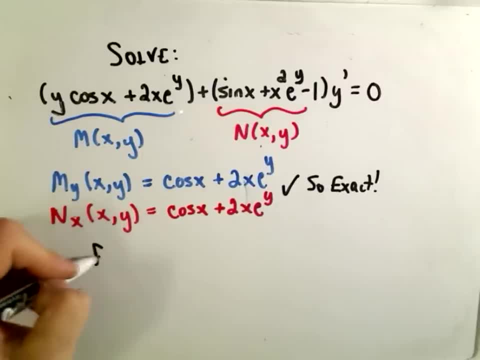 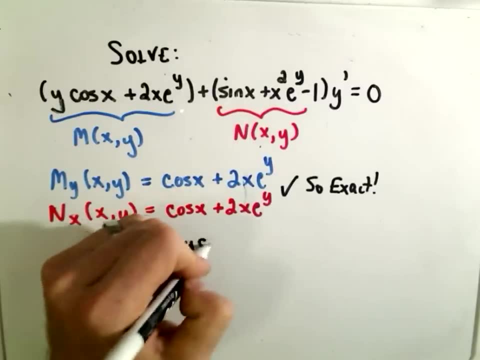 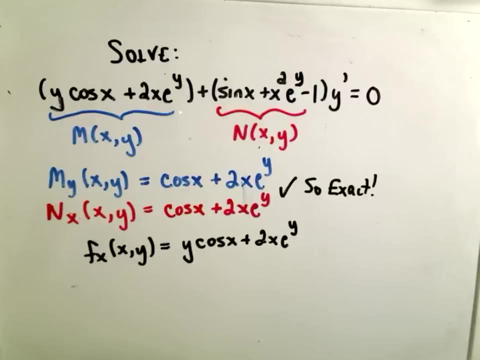 okay, so now we know that there's a function, there's a partial that equals the function, the m function, which in this case is y cosine x plus 2x e to the y. Well, if we and the other thing, excuse me, 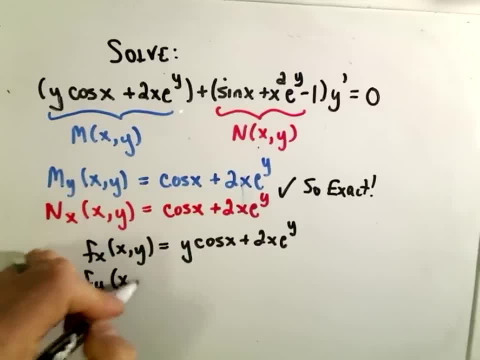 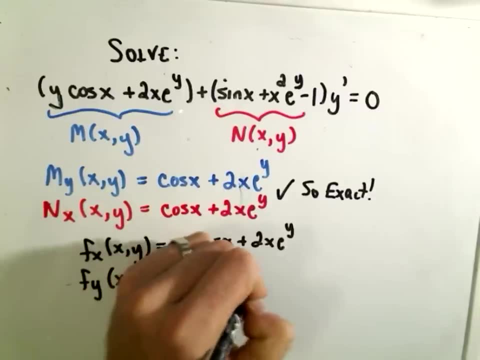 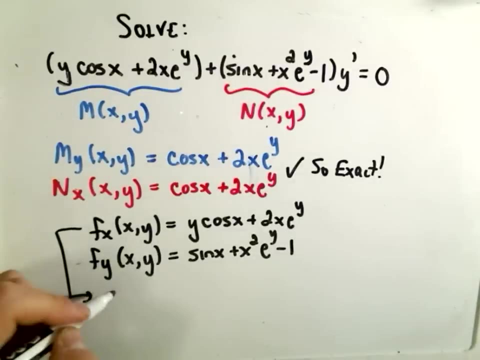 we also know there's a partial with respect to y of that function. that equals the other part, Sine x plus x, squared e to the y minus 1.. Okay, so if we take this first function and integrate it with respect to x, 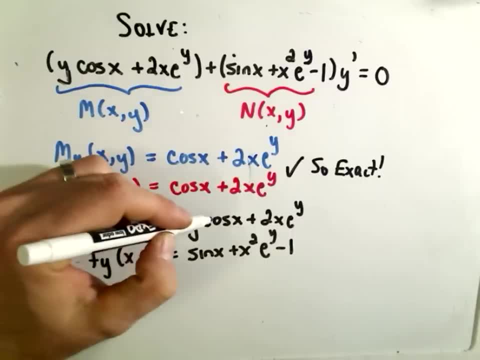 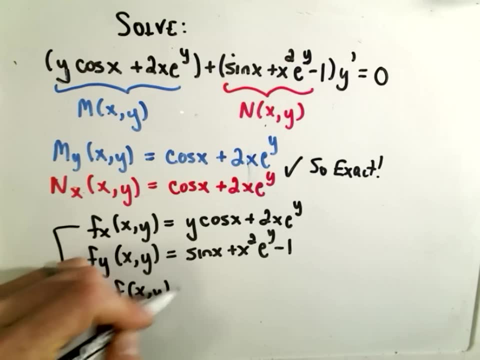 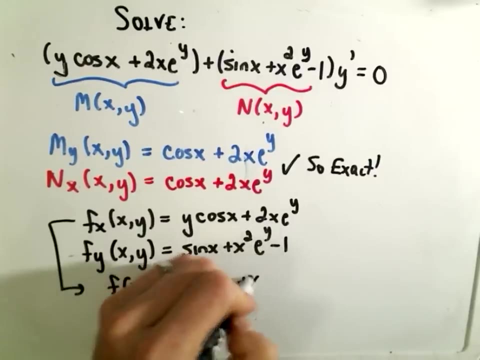 we'll get simply so if we integrate- excuse me again- with respect to x. so we're integrating cosine. so the f function, the f of x, y, we'll simply get y times sine of x. If we integrate 2x, we'll get x squared. 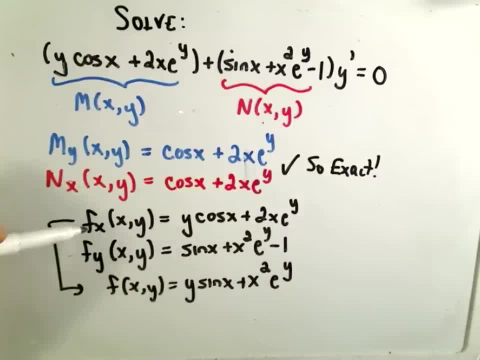 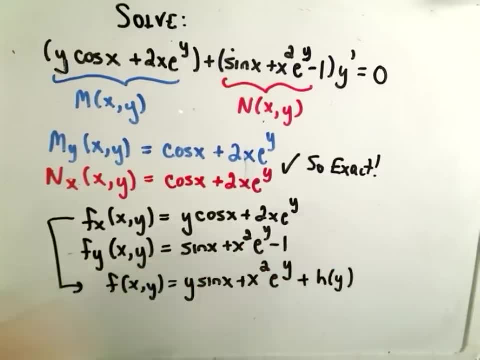 e to the y will come along. But again, excuse me, we're integrating with respect to x, so we'll have to add on a generic function in terms of y because, again, if we take the derivative of this with respect to x, 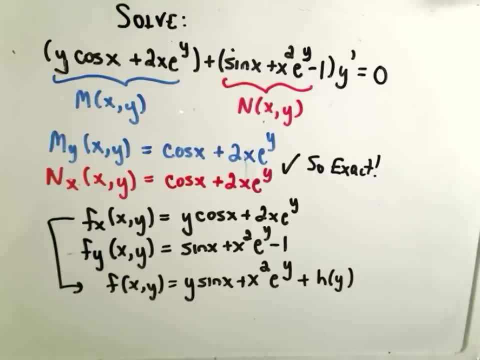 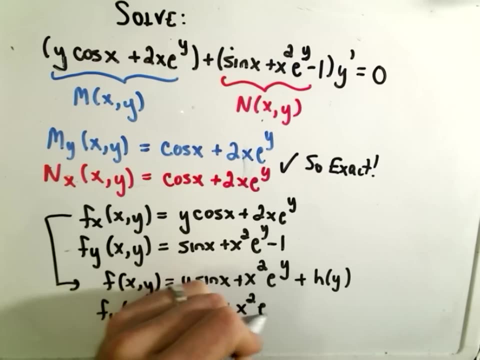 it'll simply go away. Okay, now the next thing we know is if we take the derivative of this with respect to y, okay, so the derivative with respect to y would be sine x. Again, the derivative of e to the y is just e to the y. 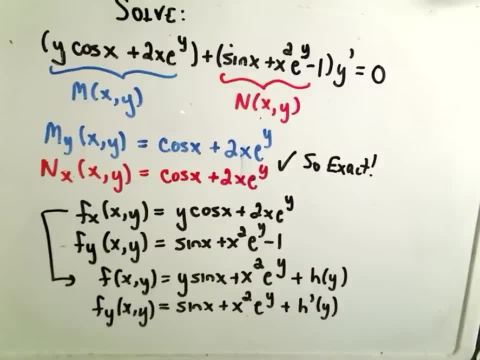 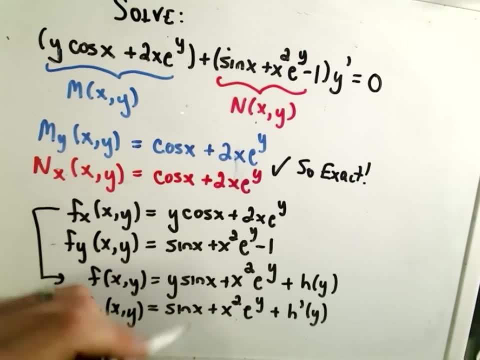 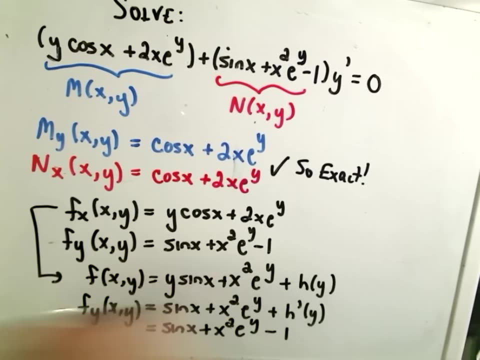 Well then we would get plus h prime of y And recall that we now know that this function has to equal the n part, which is sine x plus x, squared e to the y minus 1.. Okay, so now I'm just using this condition.